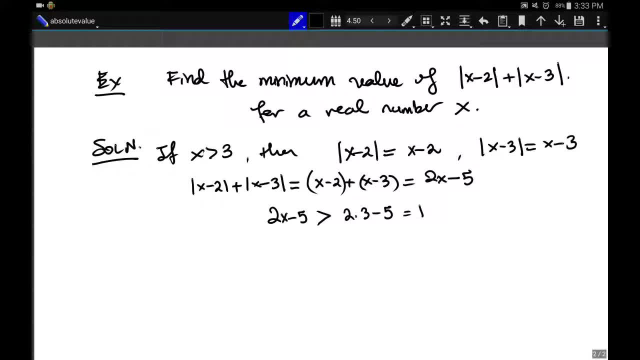 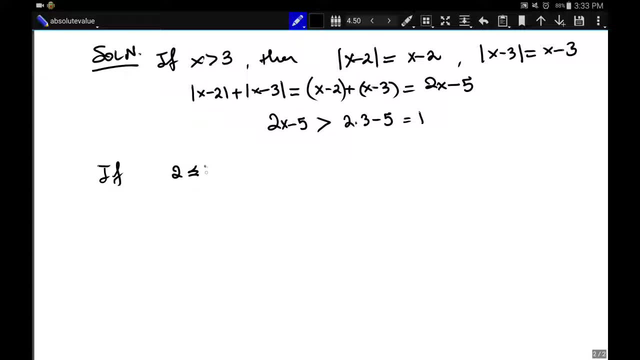 So it is 1.. So this quantity is bigger than 1.. So this is the first observation. Suppose that x is between 2 and 3. Then x is still bigger than 2.. So x minus 2 is positive. So it becomes x minus 2.. 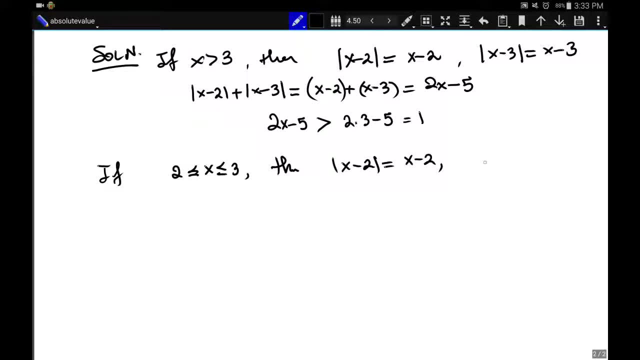 But x minus 3 is now negative because x is less than or equal to 3.. So x minus 3 is equal to 3 minus x When x is 3, so it is 0.. When x is less than 3, it is negative. So it makes sense. 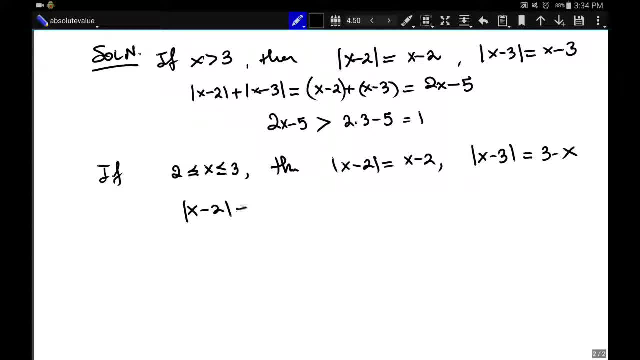 So when we add this to x minus 2 plus x minus 3.. So over here this is x. This becomes x minus 2 plus 3 minus x. So this is minus here, So this is exactly 1.. 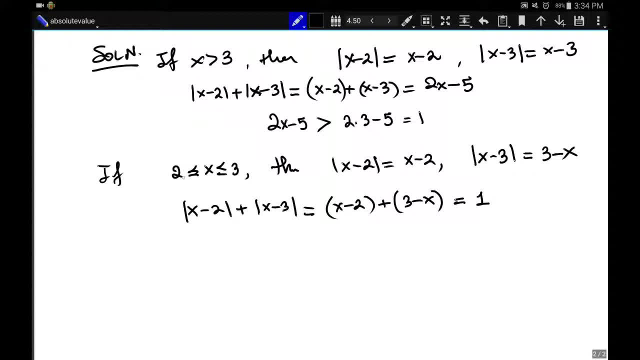 So for any value between 2 and 3, indeed, when you plug 2 in here, this becomes 1.. When you plug 3, this becomes 1.. This is 0.. So anything in between them will give you 1.. 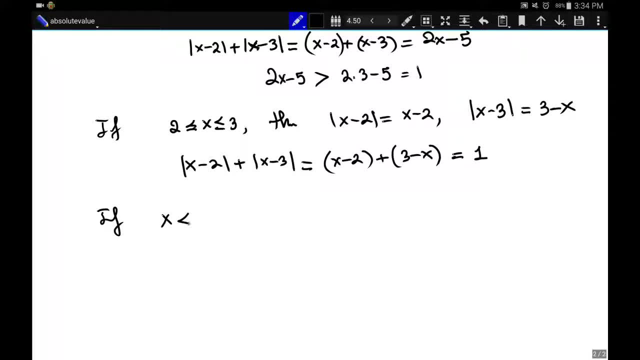 Alright, Another case. Suppose x is less than 2. Then x minus 2 is also negative, So it is 2 minus x. x minus 3 is also negative, So this is going to be 3 minus x. 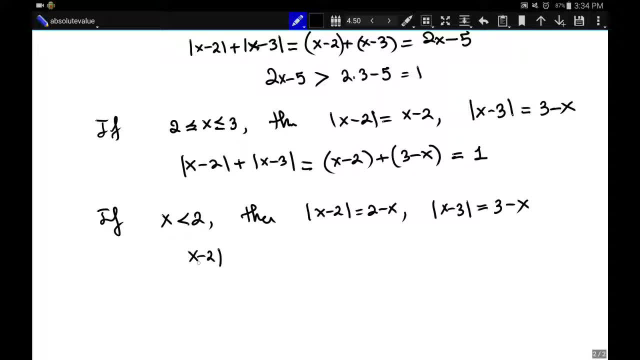 When we add them up- x minus 2 plus x minus 3 in here, So 2 minus x Plus 3 minus x, 5 minus 2x- We know that x is less than 2.. So, since x is less than 2.. 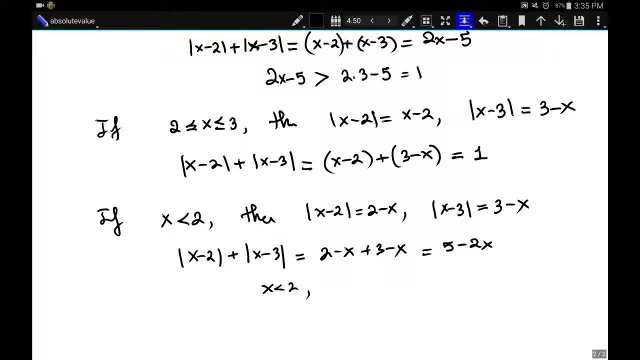 So 2x is less than 4.. And then negative 2x is bigger than negative 4.. If you add both sides, 5. So 5 minus 2x is bigger than 5 minus 4, meaning that 5 minus 2x is a quantity bigger than 1..